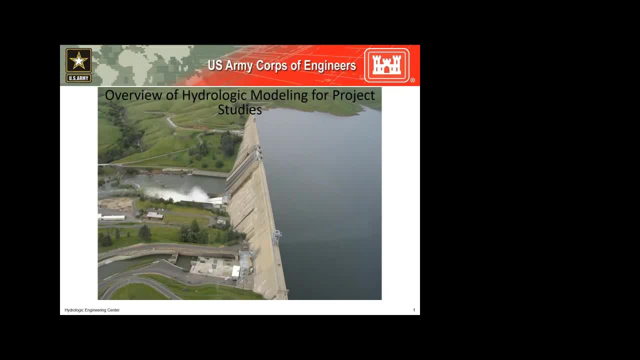 going to pay particular attention to the way that flood risk management feasibility studies are done within the Corps, but these are still applicable to basically any other study that uses hydrologic modeling. Is that Friant? That is Friant Dam. yes, Way to go, Good one. 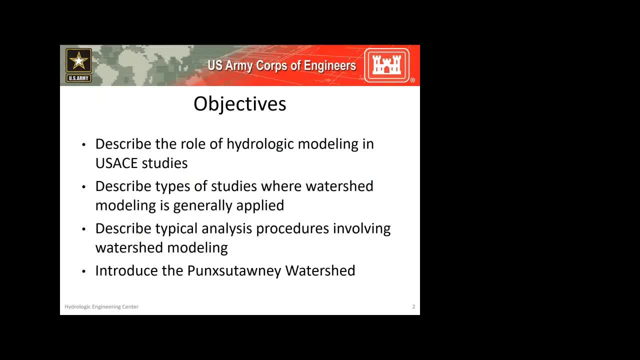 Within the presentation we'll talk about the role that hydrologic modeling plays. It's not just to model just for modeling- though I do love to model just for modeling sake- but we typically have to have a reason to expend money and time right, And we'll talk about some types of study where we do. 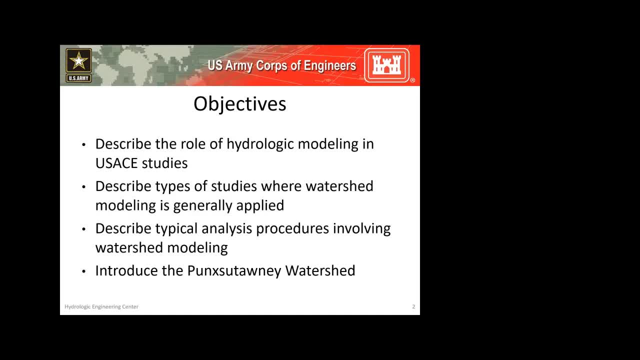 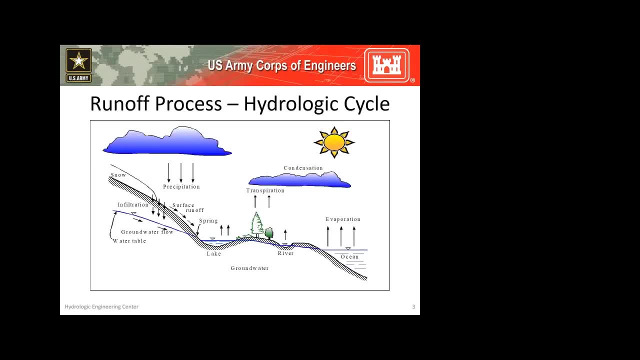 hydrologic modeling, talk about some of the analysis procedures that we go through, and then I'll also introduce the Punxsutawney Watershed that you guys are going to use for the rest of the week. There's a cartoon going through the hydrologic cycle. If you haven't seen this, 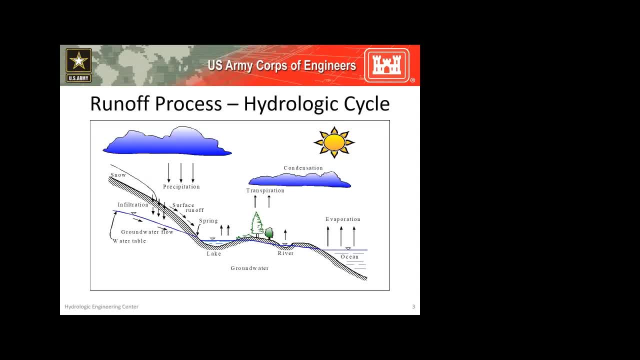 before. I'm sure you have seen this before. We'll start with water that is in the ocean or in rivers, or in lakes, or in the surface, whatever is going to be evaporated and transpired through plants. then it's going to condense in clouds. it's going to travel all throughout the 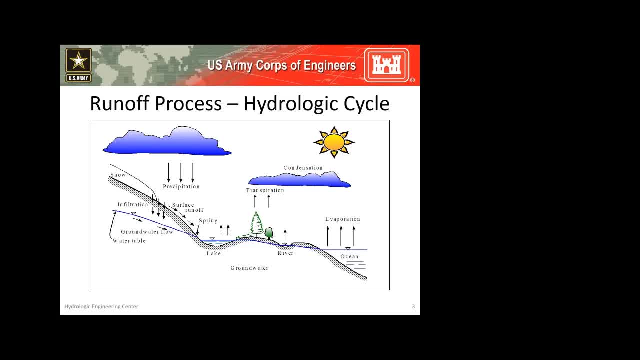 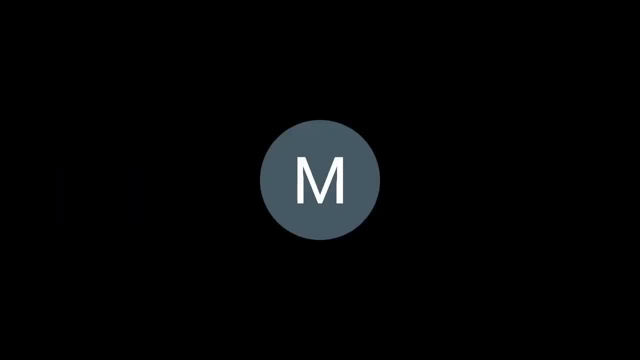 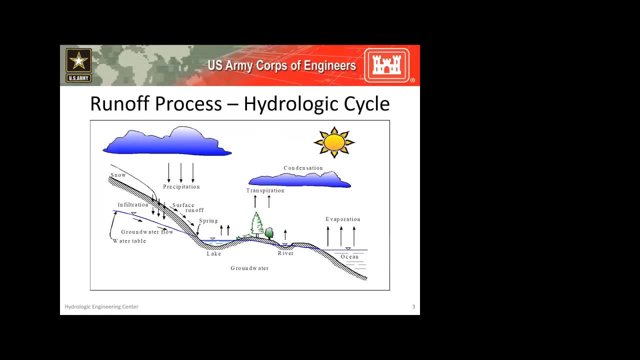 the all throughout the globe right, and then it's going to fall, as either rain, this is, so they can run off on the surface and go a whole bunch of different ways. groundwater is going to seep into the oceans, rivers and streams. anything that's left on the surface is run off in general and go into lakes, rivers and streams. 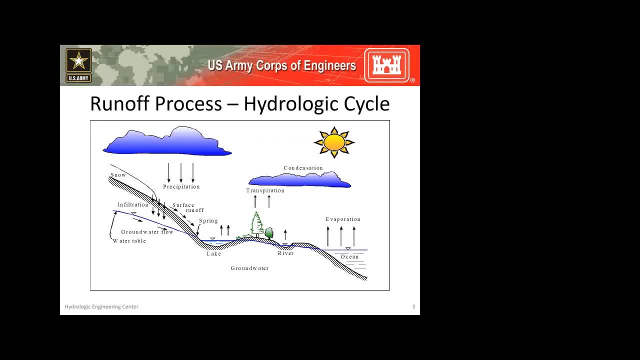 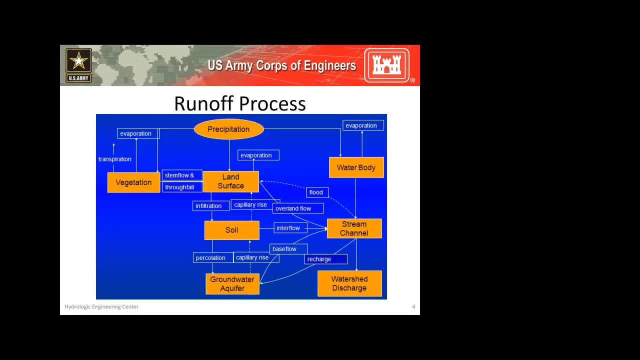 carried back to the ocean. the whole cycle starts over again, right, all this stuff is going on at any given time. we break this down within hms and pretty much any uh modeling system or application is going to break this down into a set of steps that can be followed in a time step. 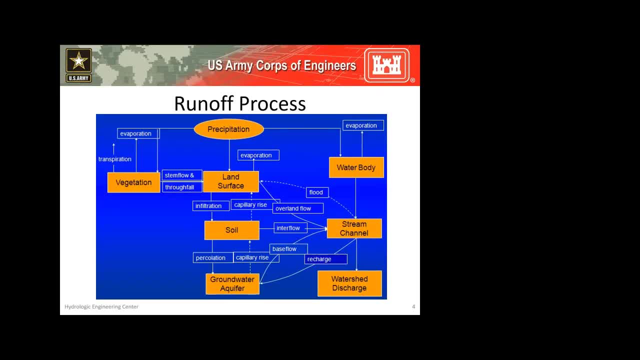 what is precipitation doing in a time step? what is the lancer in a time step, patient doing all these things, detailed than others, and each of the lectures that we're going to go through in the future, and all the workshops and everything else you can do. we're going to break all these. 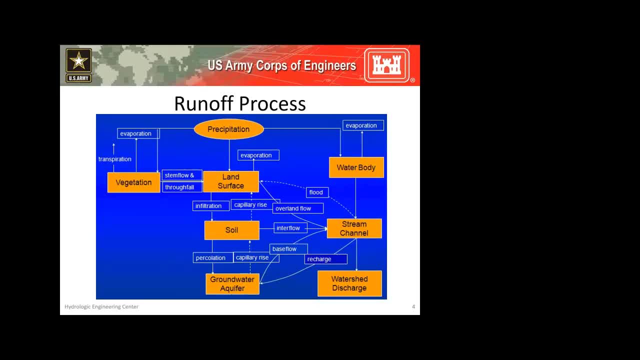 out into individual components. everything is going to be discussed. first we'll start with this, then we'll go to that, then we'll go to that, then we'll go to that, then you put it all back together again in the final project, which is really going to be cool, combining everything. 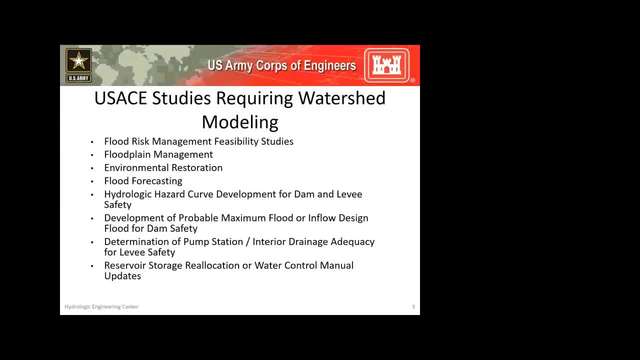 putting the discharge from a watershed, which is typically what we want, these types of studies for which we do watershed modeling, planning and designing new flood risk management facilities, dams, levees, stuff like that- typically after the fact kind of organization. so we're not doing this before bad things have happened, we're usually doing this after floods have happened, right. 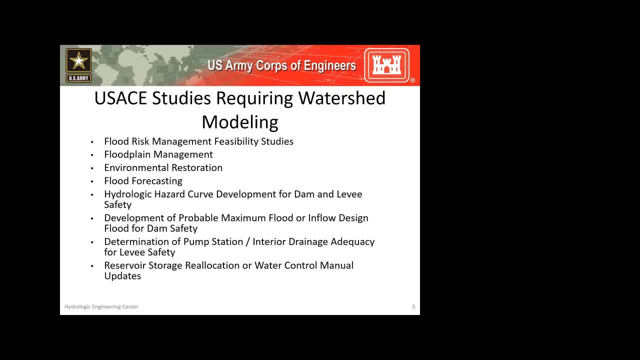 we do need to operate existing um structures like dams and levees and things like that, for flood forecasting. so we have the responsibility that usace has responsibility for operating over a 700 reservoirs throughout the country, structures throughout the country, flood control, water supply, hydropower generation. 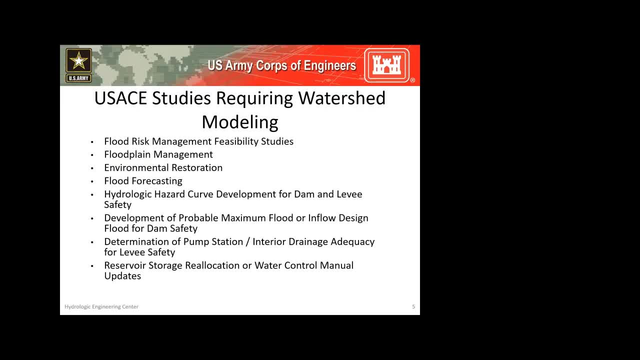 fish and wildlife protection, things like that, all sorts of stuff. um, and trying to prepare for floods would do you know? emergency preparedness activities, emergency response, things like that, regulating floodplains? yeah, sorry, sorry to butt in um, do you mind checking to see if your vpn is on? 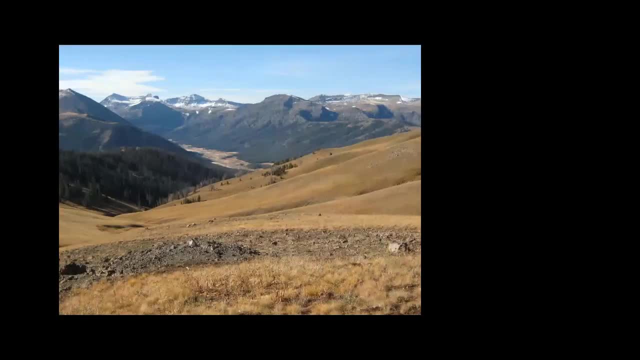 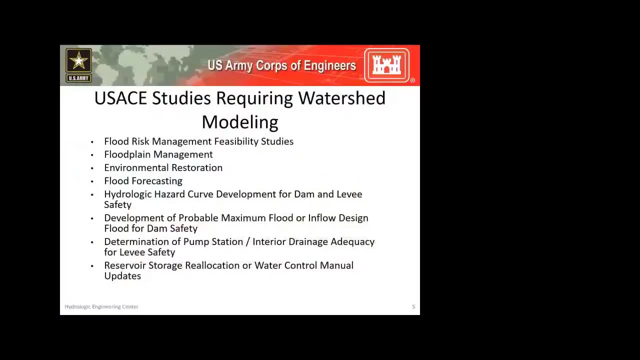 am i lagging? yeah, a little bit. it pauses every once in a while. i do not have vpn on now, oh okay, but i am at home, so subject to the whims of at t. i'm sorry. that is the only choice in my neighborhood, though. i was very happy when i moved from philly, so i came from the philadelphia district. 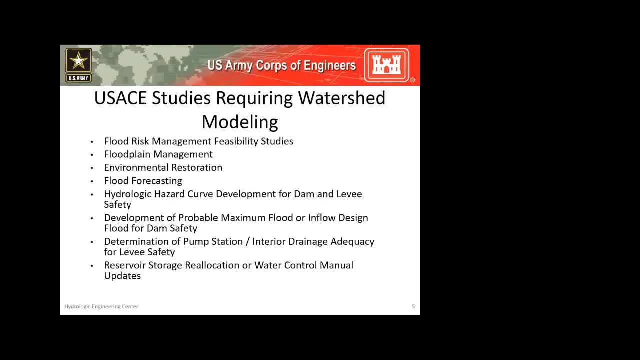 um grew up in pennsylvania, not too far from uh, where we'll be looking for the punxsutawney river or uh, mahoning creek and punxsutawney watershed. um comcast was the biggest show in town, for sure. that's where comcast got to start. i am very not have to call comcast once every six months to. 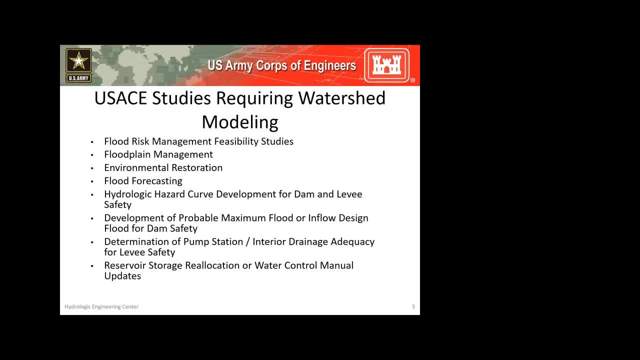 haggle and bargain on my internet plan anymore, so that's kind of nice, though it does leave me with slower speeds. hopefully we're caught up. are we on usa studies requiring watershed modeling slide at this point? yes, yeah, okay, all right, let's keep on going. then go to the next slide, hopefully our typical flood risk. 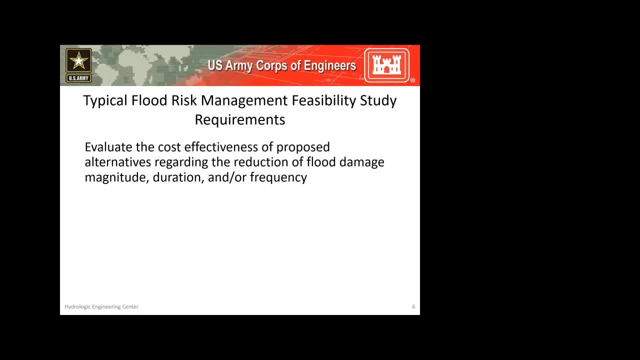 management feasibility study requirements when we're doing studies like this. um, as a taxpayer, i want to know that what you're building out there, who anybody, whether it's a state agency, federal agency, whoever local township- what you're building, uh, is it going to be cost beneficial? 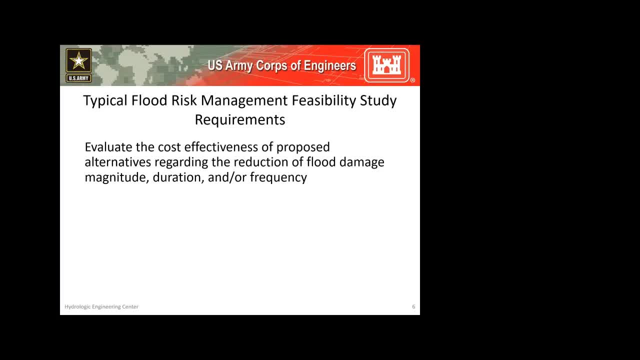 so we need to evaluate the cost effectiveness and propose alternatives. right, are you spending my dollars most efficiently? that's what we're charged with doing within the core of engineers. right, we need to evaluate how these things work in terms of magnitude, duration or frequency. right, this? this is a very simplified uh diagram to go through this, but 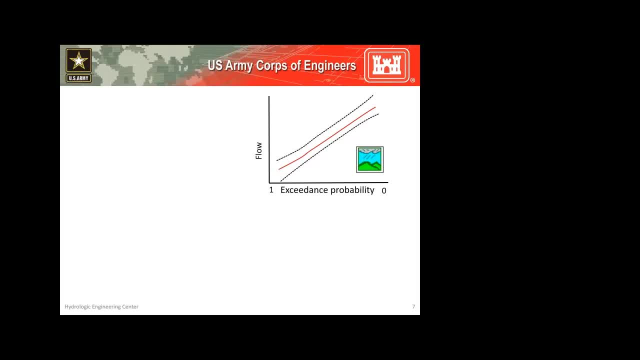 we can add complexity down the road. this is basic class. let's start simple. we're going to devise flow frequency curves or a flow frequency estimate from hc hms. we're going to start with an exceedance probability and get the corresponding flow crossover to razz, and we're going to do: 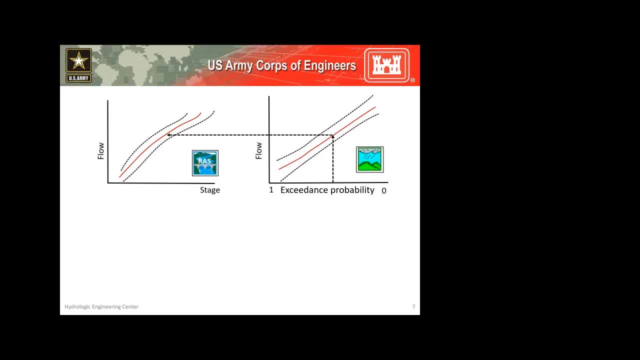 our conversion of flow to stage and inundation. right. given that stage and inundation, then we're getting to damages, right? how are the structure, how are structures inundated? how deep are they? uh, are they inundated for a long amount of time or a short amount of time, whatever? 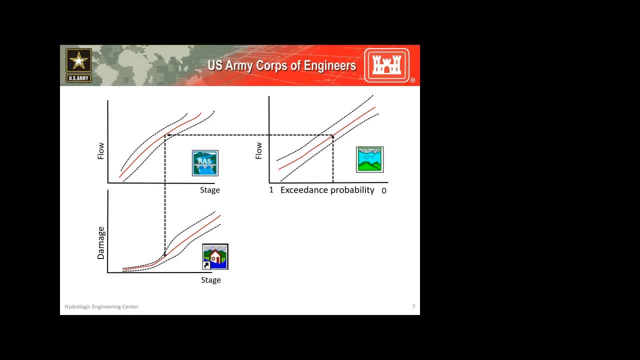 we're answering those questions in that step. given the damage from fda, fia, life, sim, a couple different, that in different ways, we'll go back to the right and for that, given exceedance probability, now we have an estimate of damage, right times we can integrate. take the difference between damages. 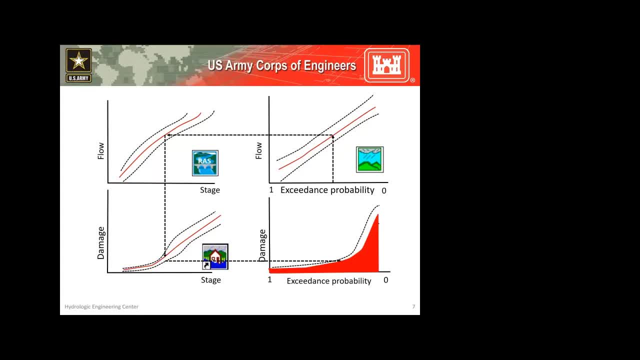 um and costs right and what we do with project conditions, then we can get it a benefit to cost ratio. we want to make sure that that bcr is greater than one. it's not greater than one. what was the point of building the project? we spent 100 million dollars building this project. 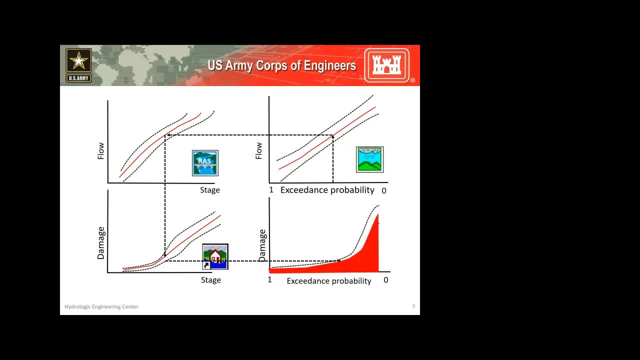 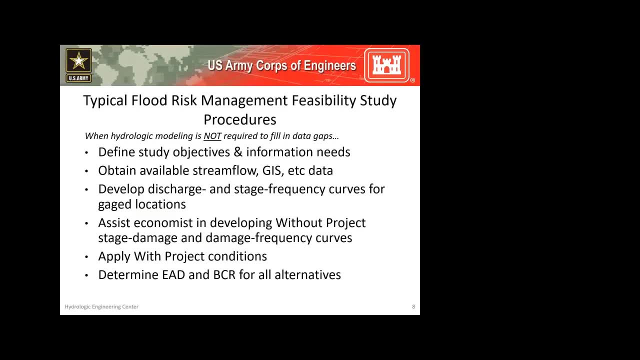 and we're only expected to get 50 million dollars out of it over its life. like that wasn't a good investment. we're trying to make sure that that is greater than one right. sometimes you don't need to do modeling, or modeling in the sense of hydrologic or hydraulic modeling, um, when you don't need to. 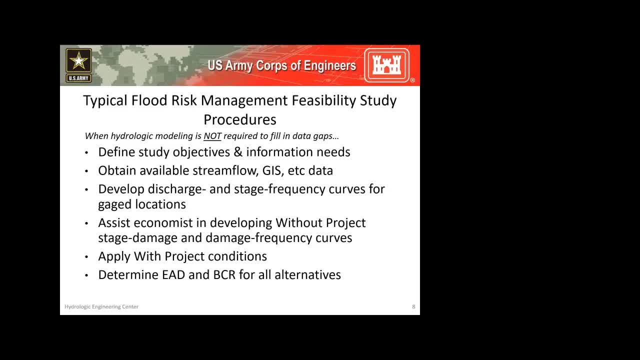 do hydrologic modeling. there are specific cases, those available. i want to grab all the available information. say, i have streamflow at the point where i actually need um, you know flow frequency or stage frequency. i have all the information available there. i can develop discharge and stage frequency curves at those. 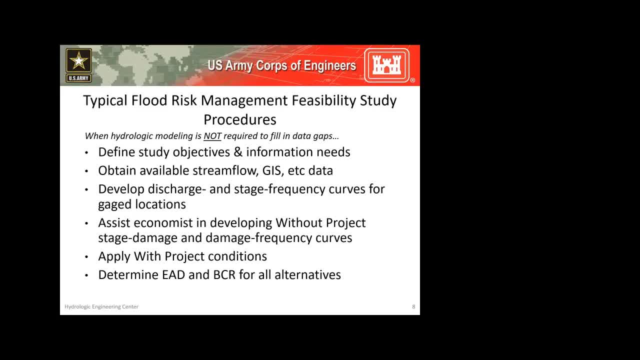 specific locations. i'll still help the economist in developing the without project stage damage and damage frequency curves, but then i might apply my with project conditions. that might be a levy or just buying structures such as your stage damage function. everything else stays the same. whatever i want to apply, those with project conditions determine ead and bcr for all of my projects. 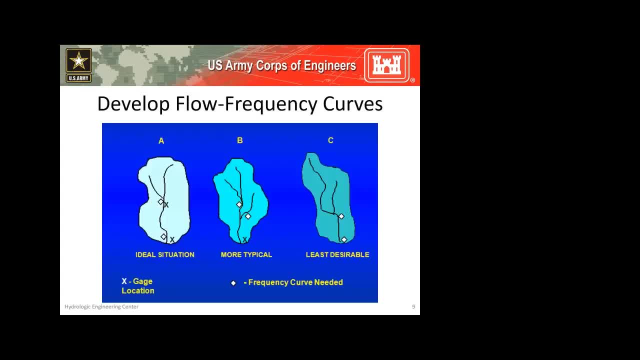 all my um alternatives and try and maximize benefits. here are the situations that you're typically presented with and when you have to develop flow frequency curves- the ideal situations on the left, right. so i need flow frequency and stage frequency, stage damage, all that stuff. i need that at the locations where i actually have a significant amount of observed. 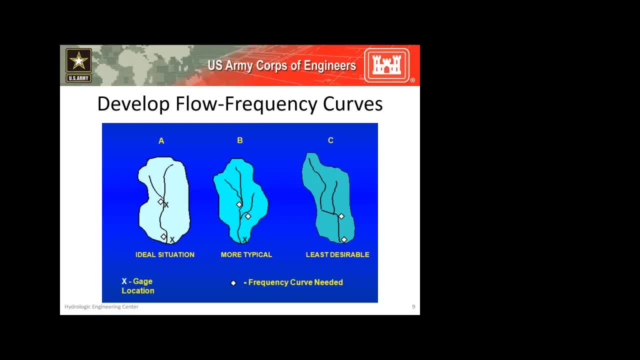 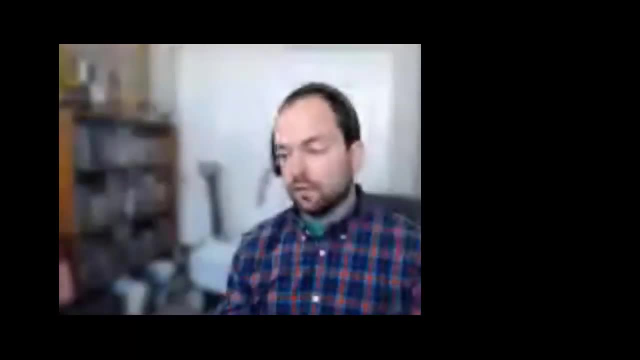 data. there might be gauges right at the towns, where i'm interested more often than not with situations either in the middle b or c where you need information as to where you actually have observed data, or there's a gauge location- um, the least desirable is on the right, but you're typically confronted with that. 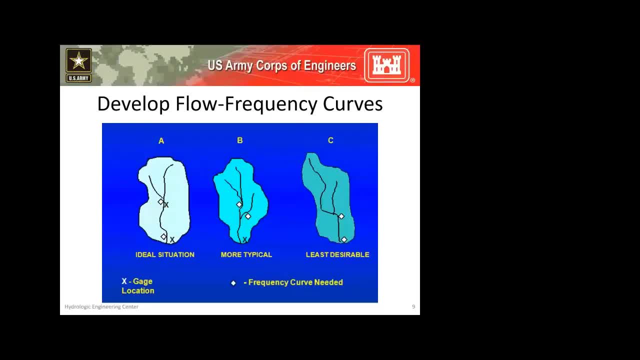 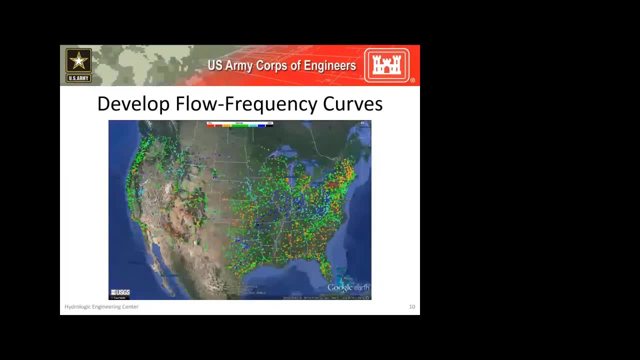 we have tools to help you doing that. there are tons and tons and tons of gauges that are operated. these are just those operated by the usgs. they are the largest purveyors of this information out there. um, fun fact: when i was undergrad, i thought usgs didn't have gauges. they didn't have gauges. 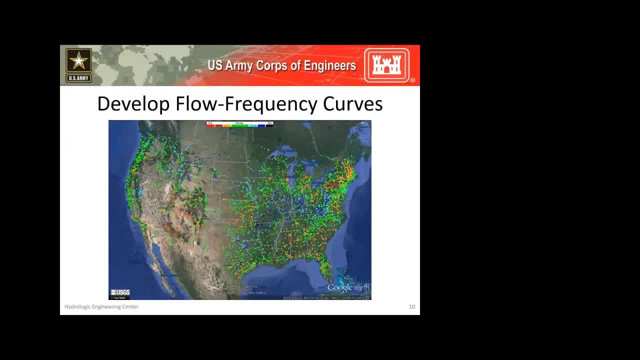 usgs, the g and usgs such for gauging, but it turns out that it doesn't stand for us gauging service. they do more than that, but anyways, they maintain thousands of gauges. these are just the ones that are active. maybe like a year ago or two years ago, whenever i pulled this information or this image, 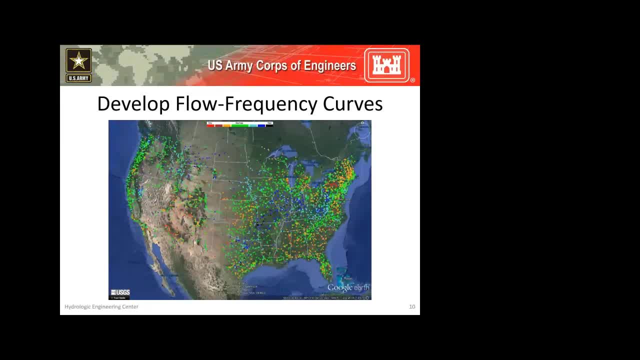 there are more and there are less. they change over time. who pays them to keep gauges in place, so on and so forth, but there's tons of these locations throughout the united states. i'm sure you guys are well aware of this when you use this stuff. 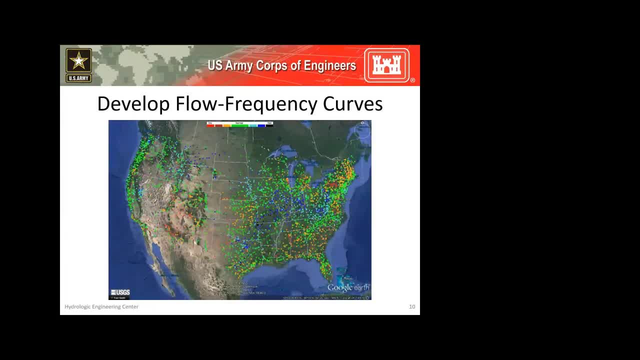 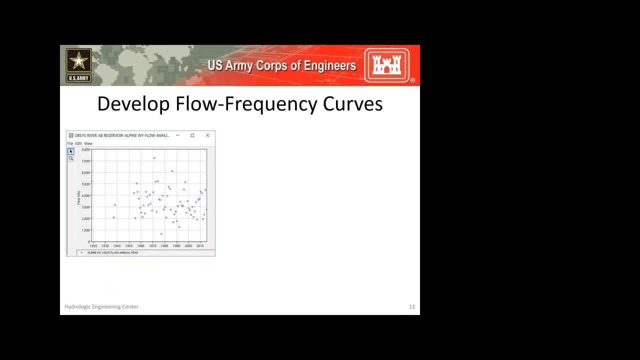 when you develop your stage or flow frequency relationships or to calibrate your hydrologic or hydraulic model. keeping going with this again, i don't need to do any more per se in terms of like hydraulic or hydrologic modeling, but i'll take a distribution like log pearson 3 apply. bulletin 17c: 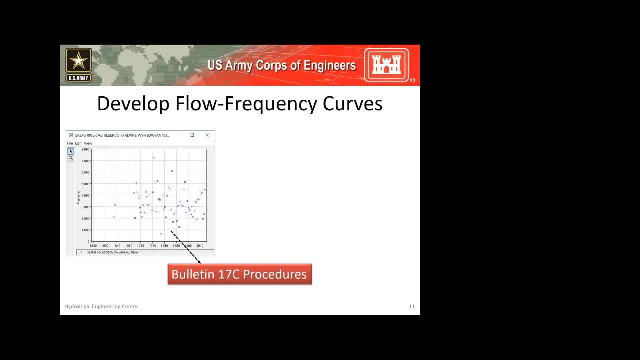 procedures to fit that analytical distribution to an annual maximum series of stream flow and peaks. i can infer flow frequency from that bulletin 17c. procedures are kind of the law of the land as it goes right now within the federal government. unless you have reason they have a catch-all. 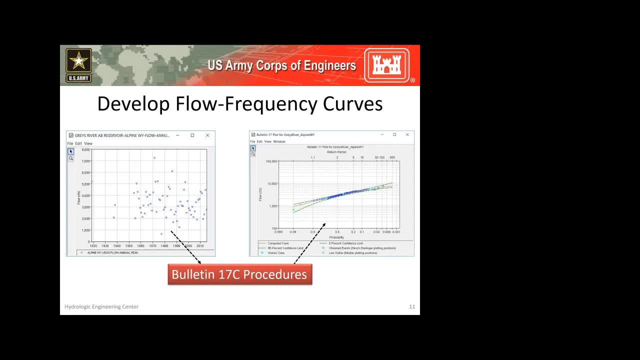 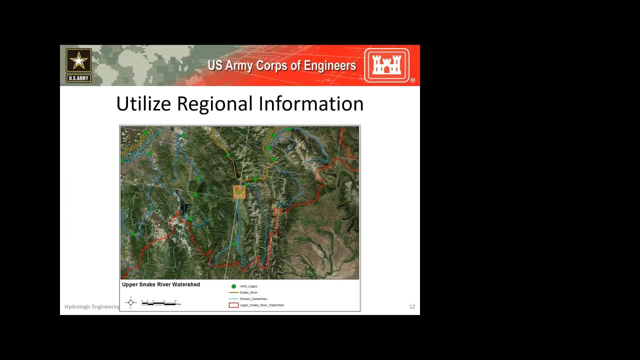 statement within there, unless you have reason to use something better, you got to prove that it's better than that. but you can do that. um, when we utilize regional information, say i'm interested in this location, this is on the snake river watershed or within the snake river watershed, uh. 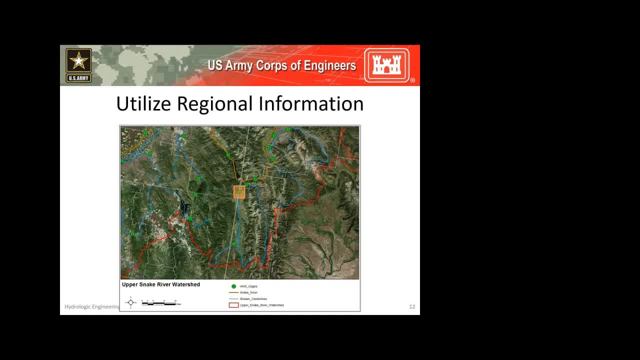 and that, let's say i have- uh, i'm looking to build a structure right here to protect a town, something like that. i might have only a short amount of, or a short time span that's covered at that specific location. i want to transfer a whole bunch of information. 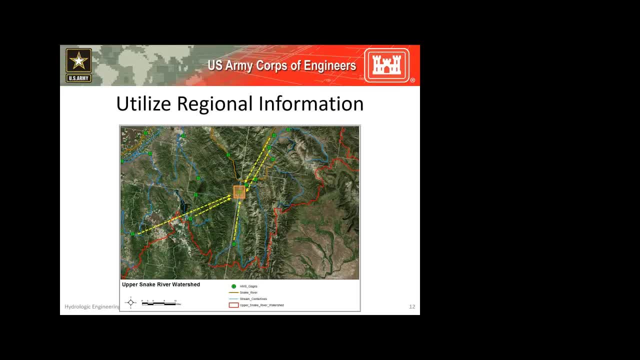 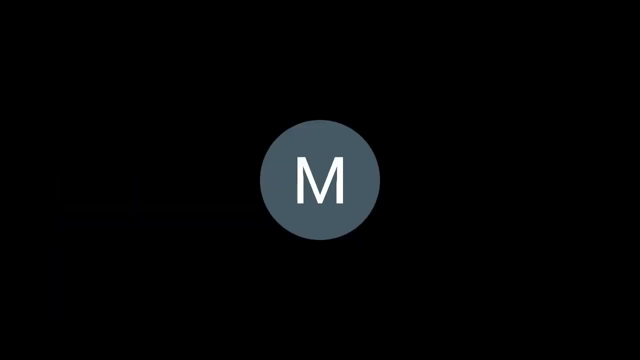 from the surrounding areas for gauges that are similar. right, i want to use and pull regional information. i can do that with statistical means like the maintenance of variance estimation, or i can use even simpler approaches like regional runoff parameters. You can even do that if you don't have gauged information, Say at this: 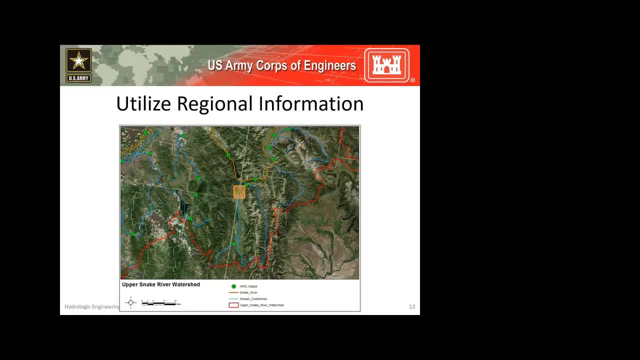 orange circle or orange box, where I'm interested. there might not even be a gauge there, but that is where I need to develop these estimates. I can still pool regional information to inform my selection of flow frequency or estimate of flow frequency at that area. But here is where 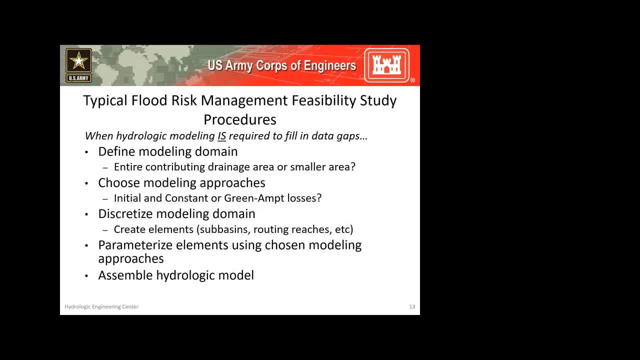 we're going to concentrate a lot of our time this week. Hydrologic modeling is required to fill in data gaps. Either you don't have a gauge at your specific location or I want a better estimate or another estimate of flow frequency. Here are some questions that you're going to have to ask. 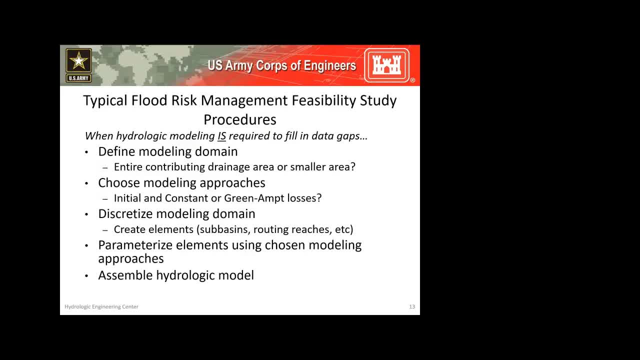 yourself. I got to define my modeling domain. Do I want to model the entire contributing drainage area or can I go for a smaller area? I want to choose my modeling approaches. Should I use initial and constant, or should I use green and amp losses? 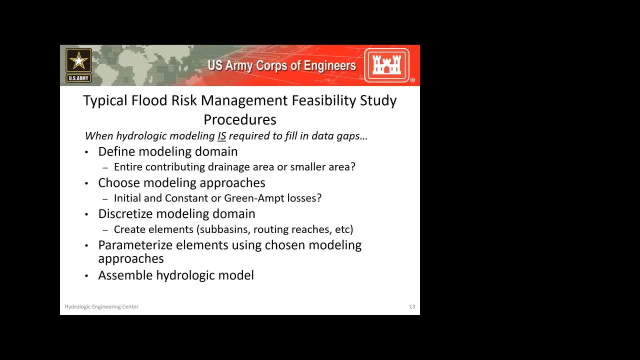 How do I discretize my modeling domain? Do I want to have subbasins, processes on the overland surface? All these questions, we're going to investigate them in detail within each one of the lectures and workshops coming up. There will be a workshop. 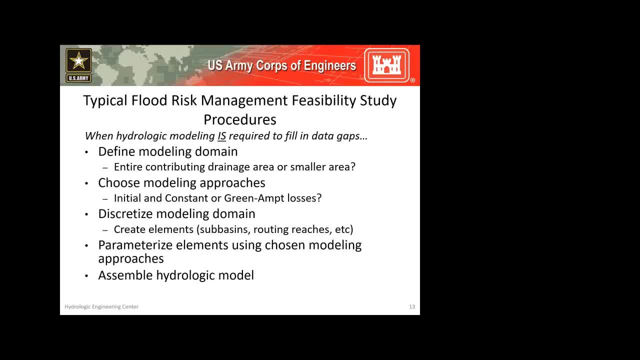 on discretizing your modeling domain. What do I do in these cases? Do I use one subbasin or three, Choosing infiltration? What's better, initial and constant? or what's better initial and constant, Or green and amped? There's a definite wrong answer to some of these questions. but initial and 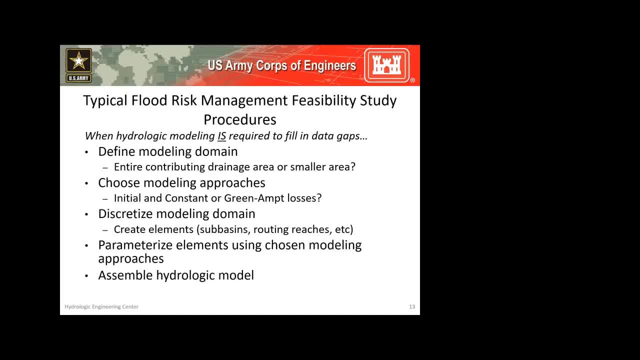 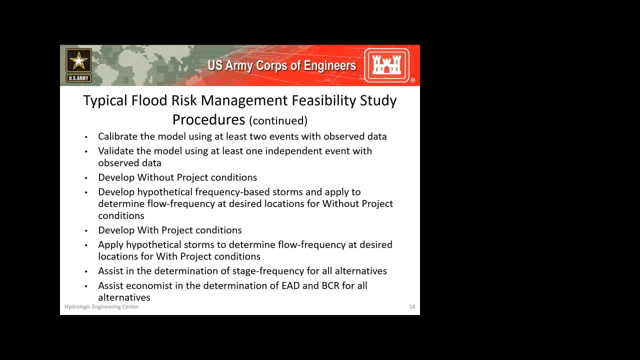 constant, and green and amped have their uses in either case. We'll go through each of those in detail. Calibration is another big one. If you don't calibrate the two events, I would leave a comment on your report and probably put that one in red and make it bold. 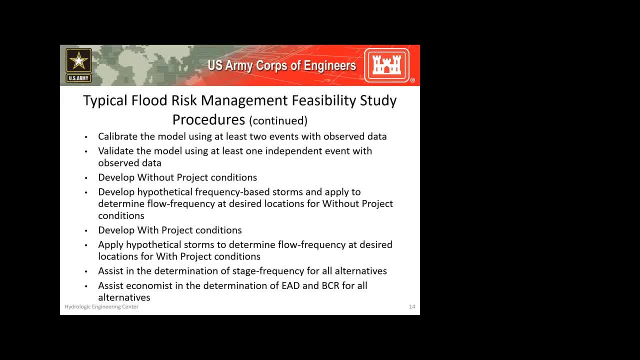 highlight it. I'm not going to let it go. I'm going to let it go. I'm going to let it go through ATR without you calibrating to at least two events. Also, you need to validate In a lot. 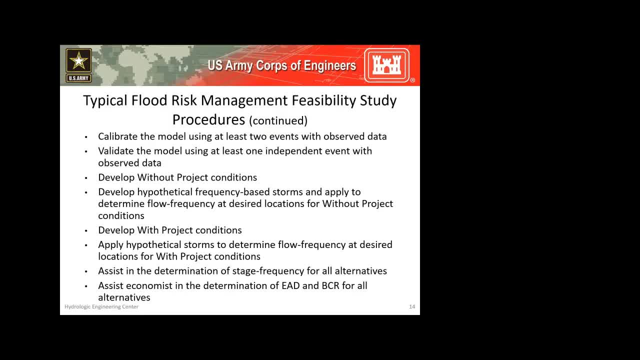 of cases, validation is more important than calibration. I want you to show me, in the absence of changing model parameters, whether that be infiltration or hydrograph parameters or base flow or something like that, when the rubber meets the road and you can't change any. 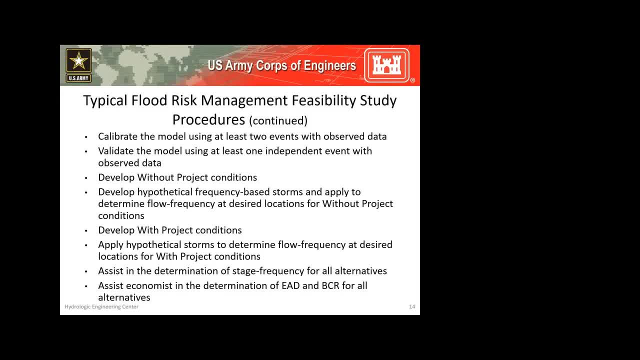 of that stuff. how well to reproduce past events. Because when you apply your hypothetical precipitation, whether that be the PMP for dam safety or the 1 in 100 precipitation for floodplain analysis or something like that, how accurate and how appropriate is your model at estimating that? 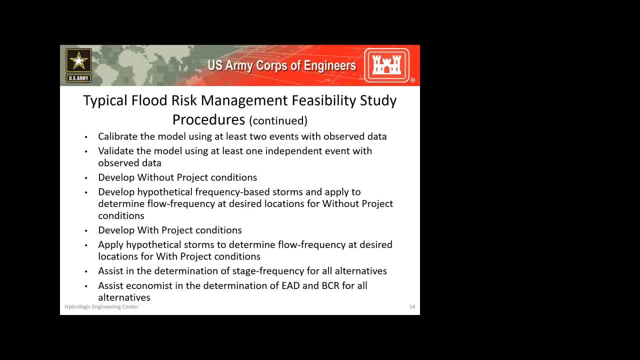 when you can't model parameters, Validation is an extremely important step. After you're done with calibration and validation, you've got to develop it without project conditions, And that's a separate bullet, because without project conditions can include something that'll happen in the near future. Maybe the state is about to build another. 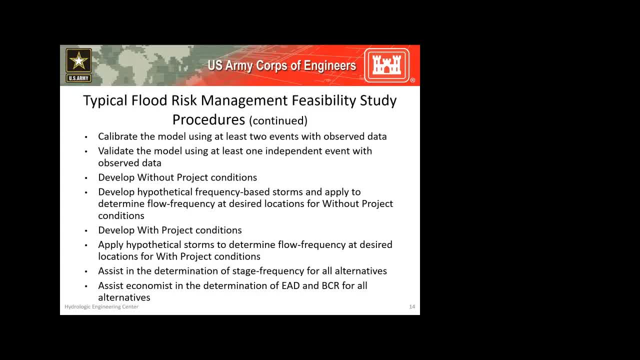 project And that's going to be online before your project comes online, so you need to take that into account. Maybe that'll knock your BCRs down below 1, and then your project isn't justified because the state got there first. You've got to develop those without project conditions independently. 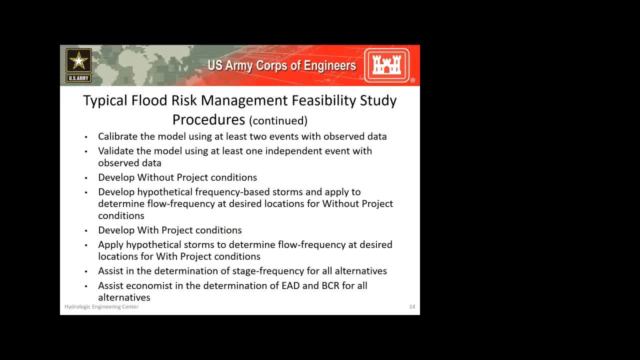 Given that, you want to develop your hypothetical precipitation storms and apply them to develop your flow frequency estimates where you need them. Develop your with project conditions. Do the same thing with precip frequency. You want to help the economist again, develop stage frequency for all your alternatives. 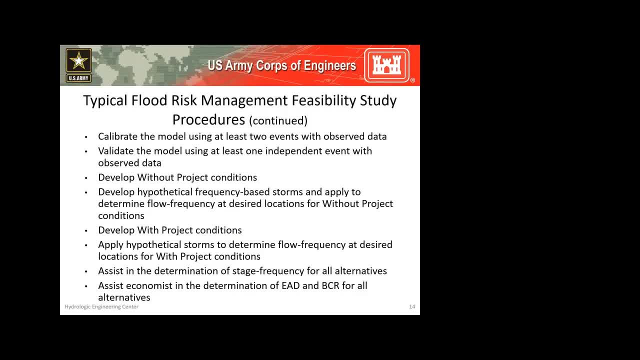 or your hydraulic guy, whoever is working with you. Typically in the Philly district we used to do that all ourselves, So I know that there are separate sections in different districts and divisions where there's a hydrology and hydraulics section. We were all in one, so we did that all ourselves. We carried it the whole way through. 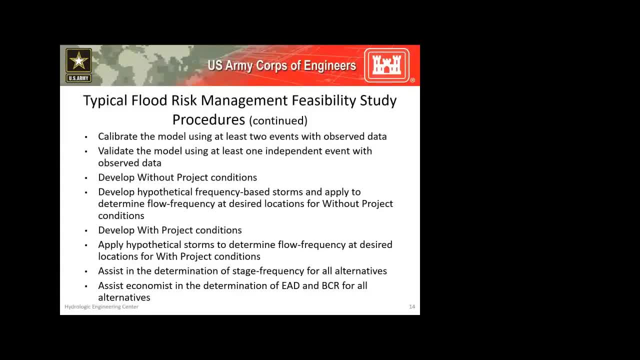 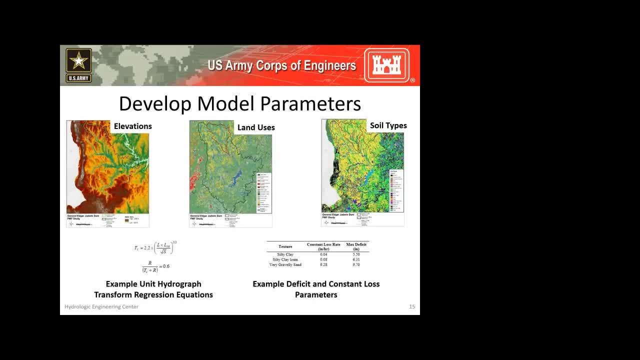 but so be it. Help the economist in the end, determine EAD and BCR For all your alternatives and again take the difference between the two. you get benefits or damages with and without project. When you're developing your model, you're going to pull a whole bunch of different. 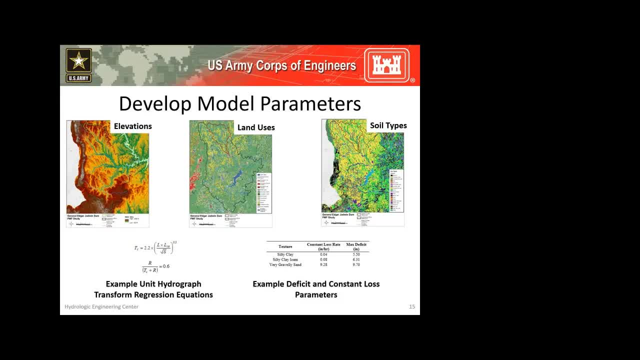 information together. Here's a couple of examples: Elevations, land uses, soil types. they're all used for different processes. For instance, elevations are going to allow me to delineate my watershed. Does water go this way or does it go that way? If it goes that way, 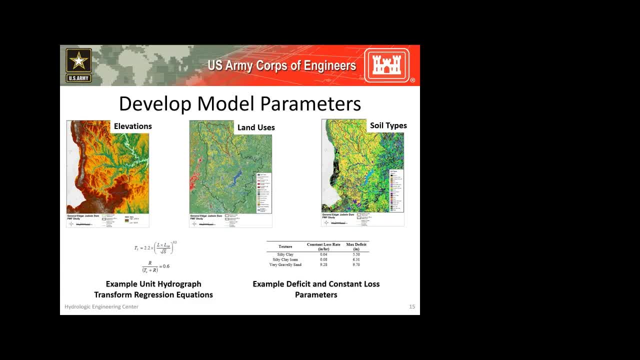 then it goes into my watershed. If it goes that way, then I don't care about it particularly. You can use hydrograph transform regression equations like the ones that I showed here, and I think we're actually going to make use of those later on in some of the workshops as well. 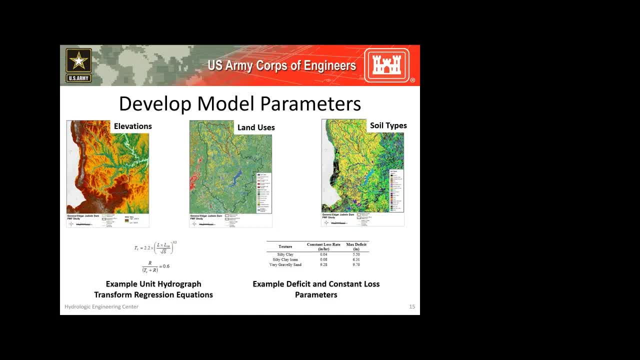 You'll see them again in the future. You're definitely going to use these relationships for deficit and constant things like that from, say, Rawls, Brackensiek and Miller for estimates of constant loss rate or saturated hydraulic conductivity for a given soil type. 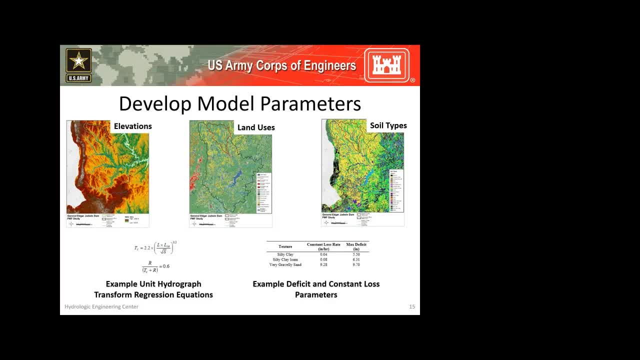 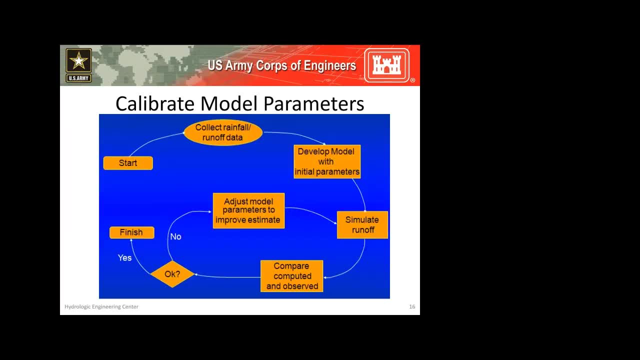 You'll definitely use those in some of the lectures and workshops for losses. Let's see these guys again. Then come to calibration. I think Tommy has a better graphic than this one, but we'll just keep with this one. Notice how it's looped. It's an iterative. 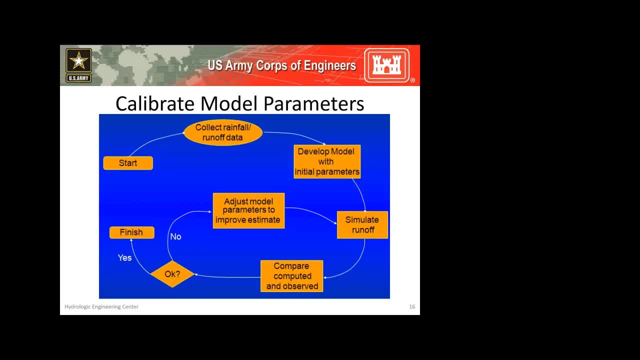 procedure. You start and you might get to a point where you're like, oh, I need to go back and I need to try this again. If you only take one shot through here and you say, all right, am I good. 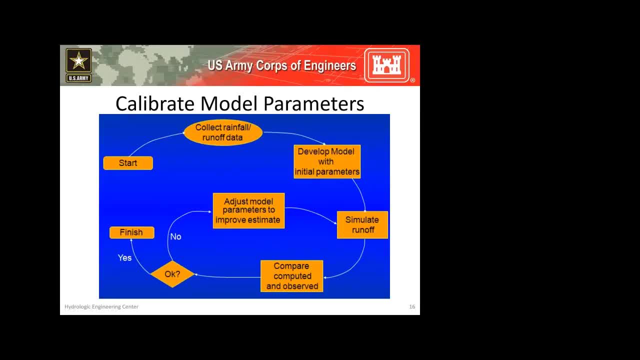 Yeah, that doesn't happen. Try again. You can always make things better. For your final project, we are going to put down some guidelines and rules and then we're going to go back and try this again. Some guidelines and rules and grading rubric that be kind of clear. You use statistical metrics. 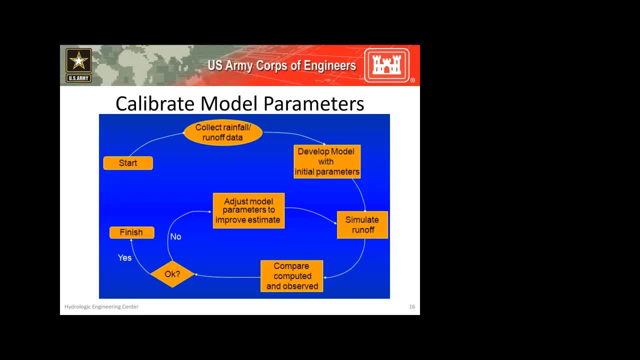 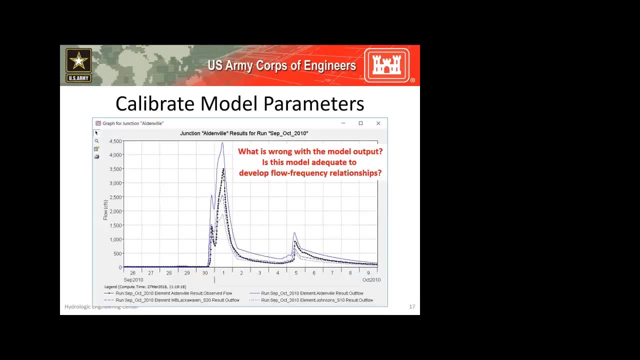 to compare how good faults are for certain national efficiencies, percent bias, so on and so forth. Does anybody know out there? Go ahead and unmute, Talk in your mic. What's wrong with this? Is this appropriate to estimate flow frequency? What would happen if I use this model to estimate? 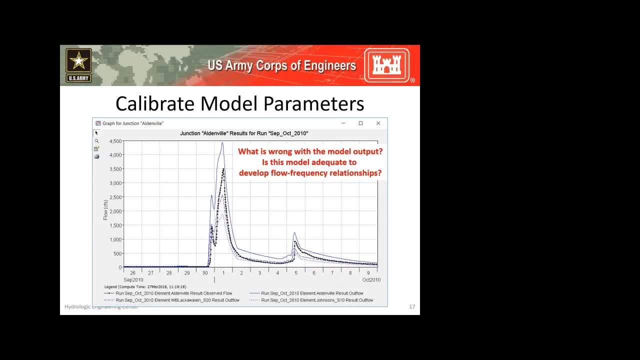 flow frequency. I want to hear your voice Tell me Overestimation. I'm sorry, say it one more time: Overestimation, Overestimation. Yeah, so runoff is overestimated. What's wrong with this? What would I do to make this better? Increase loss rates. Increase loss rates. Maybe change base flow. 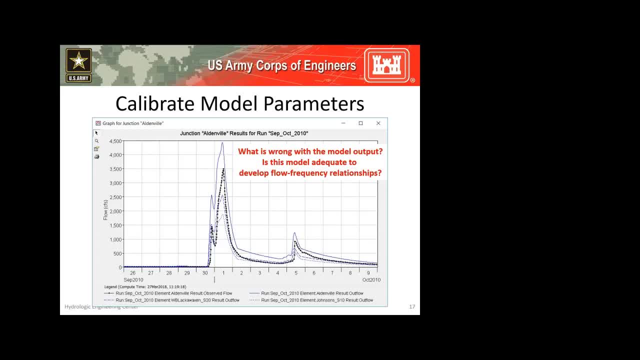 Maybe change unihydrogram, Maybe change graph transform, though the shape looks generally light, right. If I use this to estimate flow frequency, what do you think is going to happen in my flow frequency relationships with regards to the true flow frequency relationships? 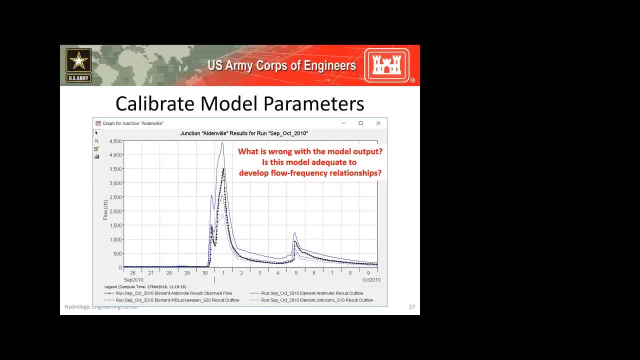 Will they be biased in any way? Be biased up, right. You'll hear me say this over and over again. That's no bueno. It's not a good thing to just be like: eh, it's close enough, but I'll be wrong all the time, so it'll carry out in the end. Don't do that. 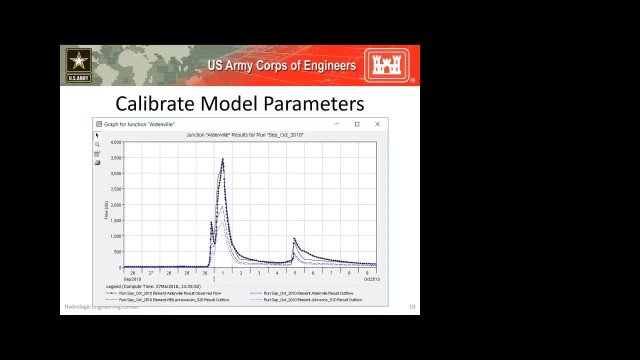 Change your parameters to better estimate what you need to use for your study In this case. look at that. I'm so much better. All I needed to do was change a couple of loss parameters or base flow, and I was better estimating what happened in the past. 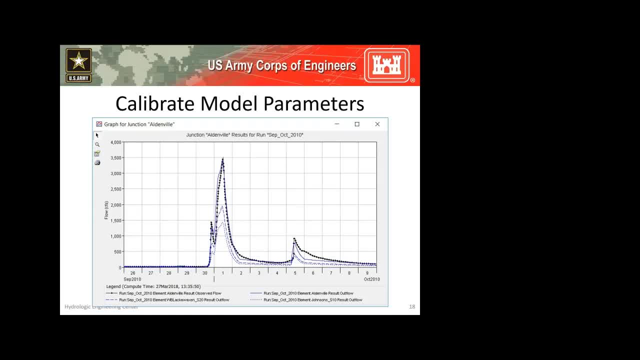 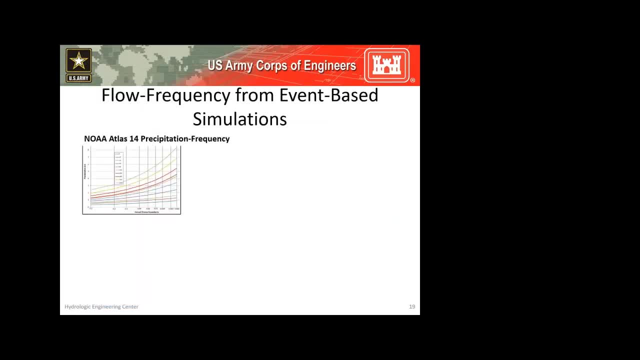 I'll do this for a couple more events. right, That's calibration. You want to do the same thing for, like I said, for a couple more events, then validate to a couple of independent events where I'm not changing parameters. Once all that's done, I'll take a simplified approach to coming up with flow frequency. 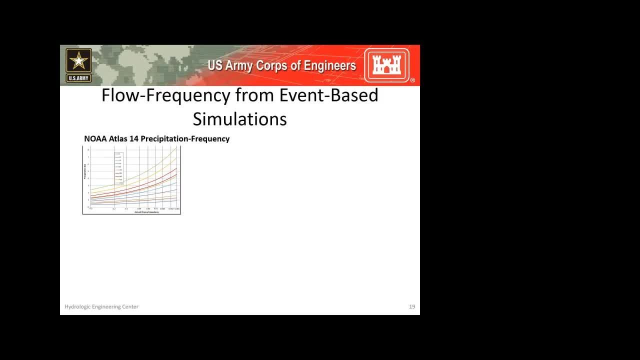 Here's one way to do it: the deterministic approach, and Greg can talk a whole lot more about this, because this is Greg's wheelhouse. in terms of developing flow frequency using hydrologic models, Some cool stuff is coming online. It's even online now. 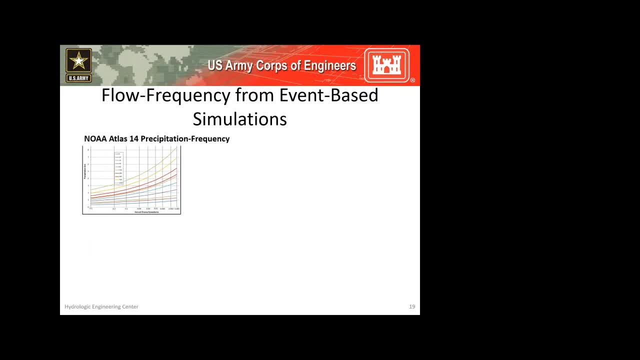 but I developed these slides maybe like four or five years ago. This was the way to do it then. Now we have automated routines to do a little bit better. I'll start with Atlas 14 precept. I will grab, say, eight different events or generate 10 different events I can generate. 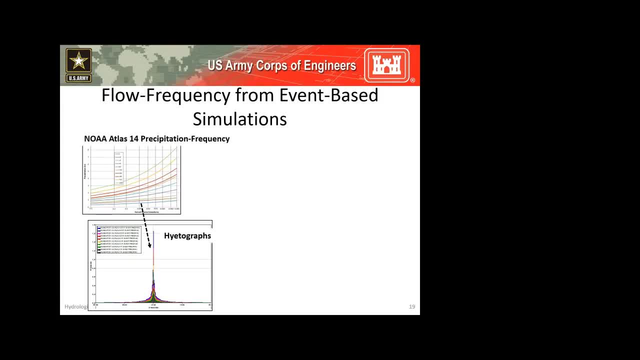 hiatographs. These are balanced hiatographs. There's some problems with that. for sure, You have the 15-minute storm within the 30-minute storm within the 60-minute storm, so on and so forth. Real rainfall typically doesn't fall like that, so maybe you want to use a different pattern. 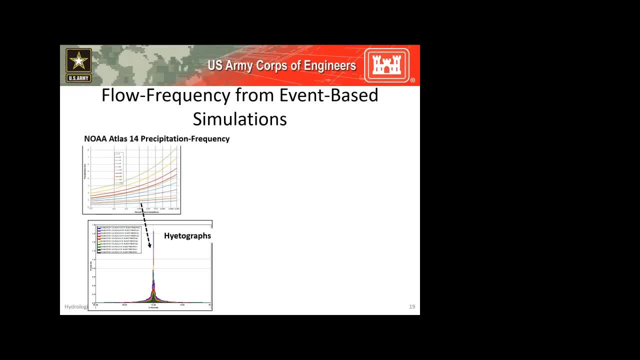 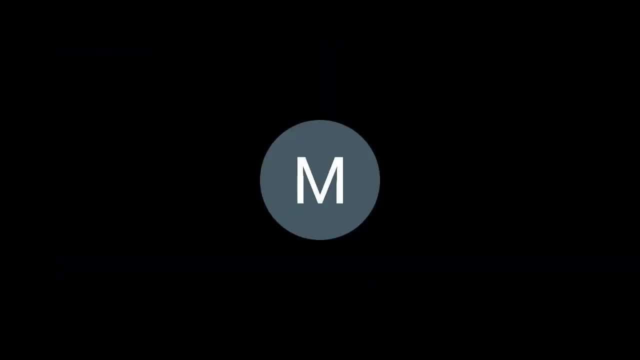 Either way, I can generate these hypothetical storms that you're going to be able to see. I'm going to go ahead and do a little bit more of this- My model- but in this case I'll grab those peaks and now I can estimate flow frequency. 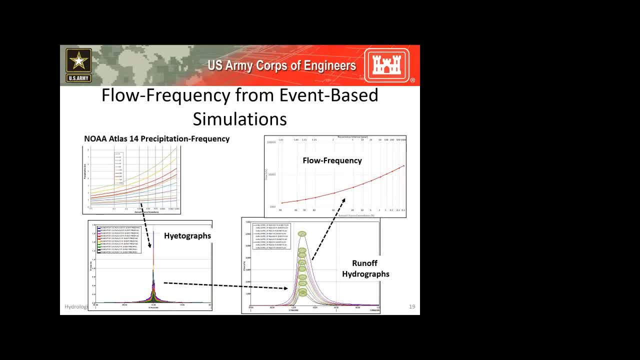 HMS can automatically do a bunch of this stuff for you. Specifically, the depth area analysis is going to adjust your storm area to give you better estimates of the hiatographs to use, and it'll automatically extract the information for you and present it to you in a usable way. 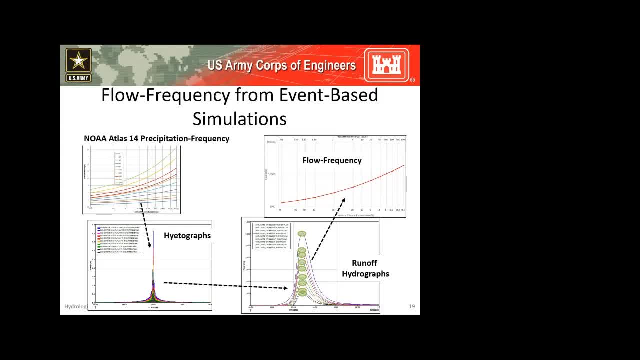 There's some really cool stuff coming online right now within HMS, or has been online. The hypothetical storm does a much better job than this. This is the frequency storm approach, the frequency storm met model. Definitely take a look at the hypothetical storm if you haven't Cool stuff coming in here. 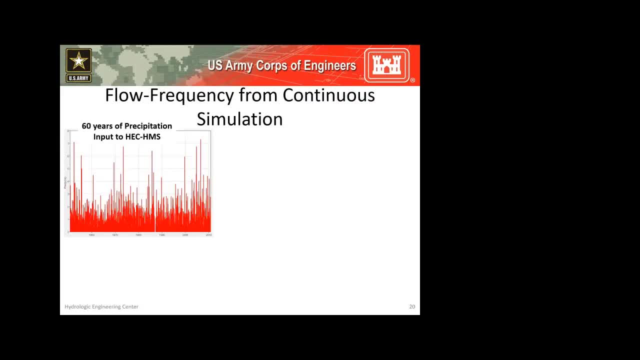 Another way to do this. instead of doing, say, eight different deterministic frequency-based simulations, maybe I just want to simulate 60 years of precipitation within HMS. I can totally do that. Take my 60 years of precip, put it into HMS and I can develop 60 years of runoff. 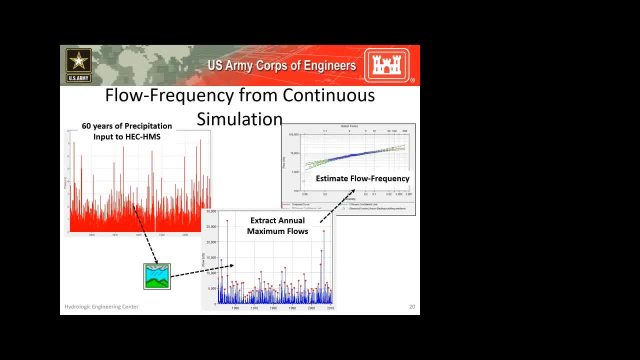 Let me just extract the annual maximum flows, and now I can use Bulletin 17C procedures again or fit another analytical distribution to that information to estimate flow frequency. Here's my estimate of flow frequency, and I started with simulating 60 years of precipitation. No hypothetical precipitation was applied in this case. 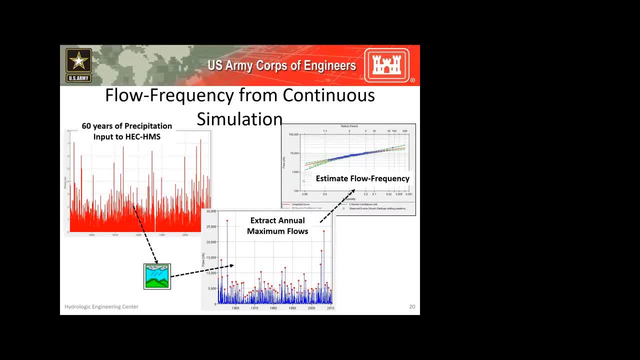 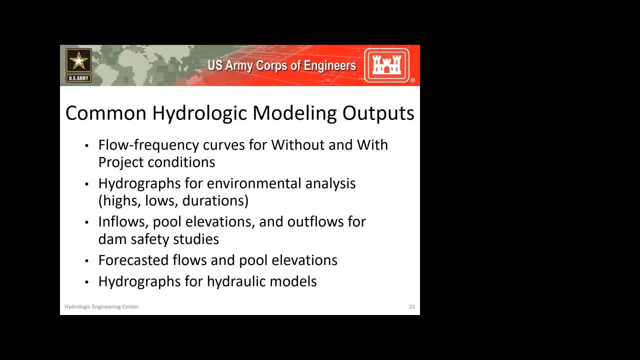 so this gives me flow frequency at that location, Some typical modeling outputs that we're going to go after when we're doing hypothetical or when we're doing hydrologic modeling- and we talked about this- but flow frequency curves, that's usually the meat. That's what we want for both. 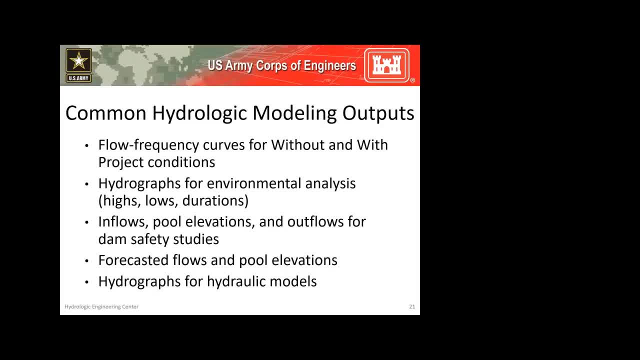 without and with project conditions, because I need to get the difference between the two to give me benefits. Maybe we want hydrographs for environmental analysis, like: how long is flow above 1,000 CFS or something like that: How deep is water going to be in this specific location? 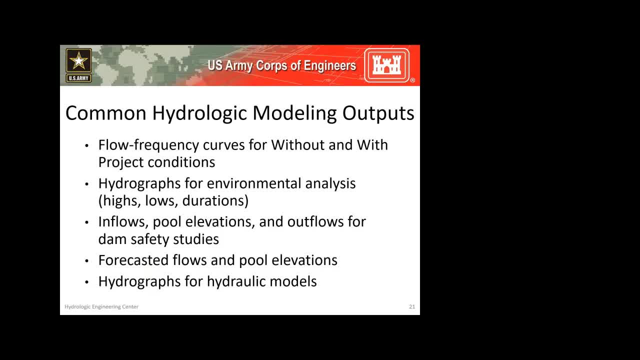 How long will it be? over two feet deep, because that might kill my crops, something like that. but I also might need inflows to a project of consideration because I might need to regulate based upon inflow and not just pool elevation, but outflows are also important. Pool elevations are important, Inflows are important- All. 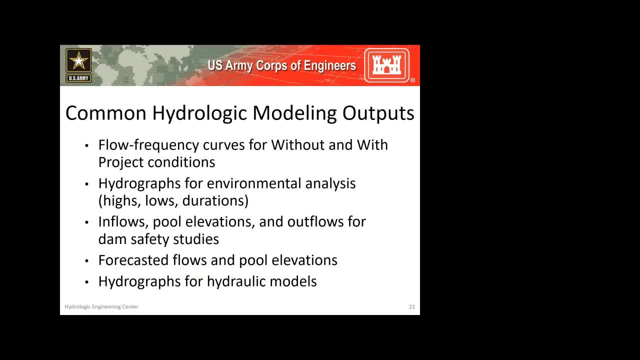 gamut is important for dam safety, Forecasted flows and pool elevations, so sometimes you've got to flip the dime over and be like: well, now I'm not interested in taking six months to answer this question Now. I only have 15 minutes right. So that's forecasting. 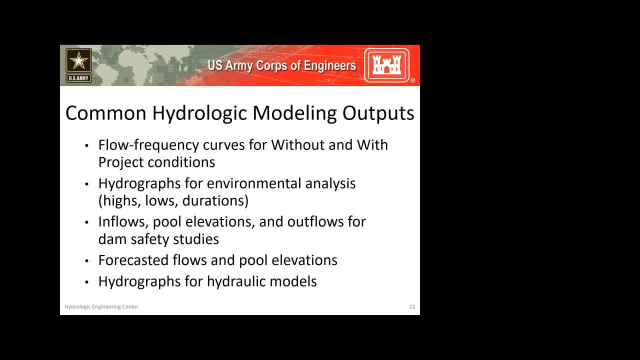 in a nutshell: I've got to do it quick. How accurate can I be in the future? Now I need to be fast with it. You also need hydrographs for hydraulic models too. We're kind of blurring the lines between the two. Definitely made this slide a long time ago. 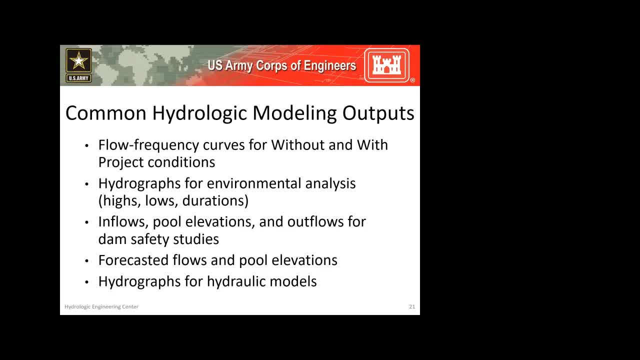 because you can do a lot of these processes within either RAS or within either HMS. You can carry things all the way through and get a complete picture of it. We'll keep doing that in the future. give you guys more options. Definitely want to say that there are guidancegov. 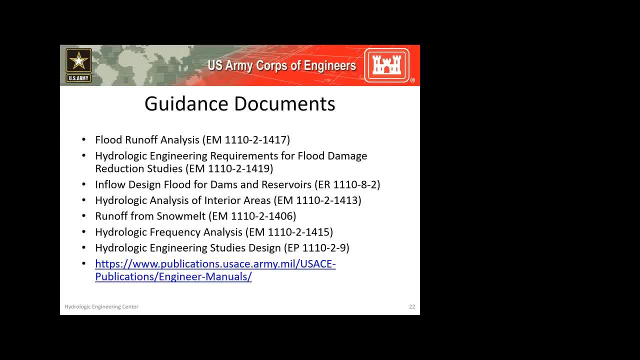 if you're looking for guidance on how to do this, there's a lot of documents out there that define how you need to do these things for the Corps of Engineers right. What is an acceptable modeling practice when doing a flood risk management feasibility study? Those things are all lined. 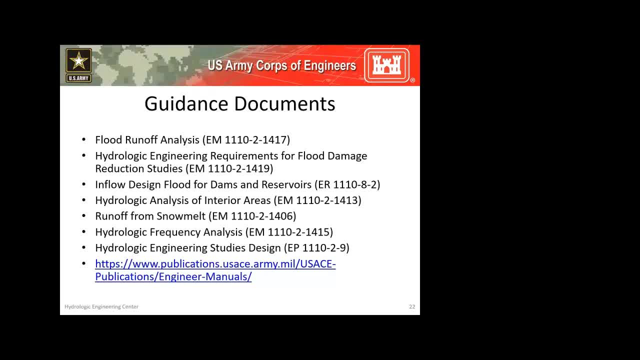 out here. There's publications that are available that are pertinent to these discussions. If you haven't, go to this publications website where EUSASE keeps them all. This is just the engineer manuals one. There's also one for engineer regulations, So on and so forth. They're all there. They're available for discussion. If you haven't. 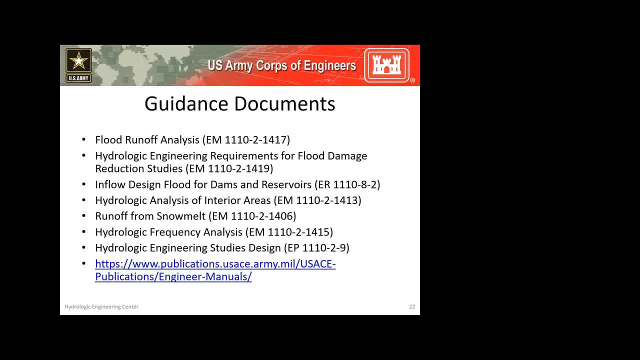 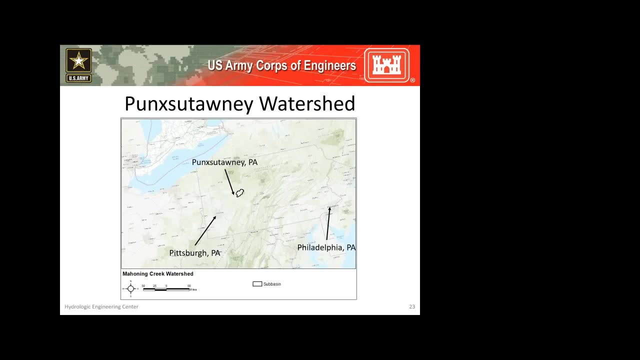 grab them, take a look at them. They're kind of dry to read, but there was a lot of time spent in developing those and laying things out on how the Corps will do these things. All right, let me take a step back. Let's talk about the workshop watershed. Here is where 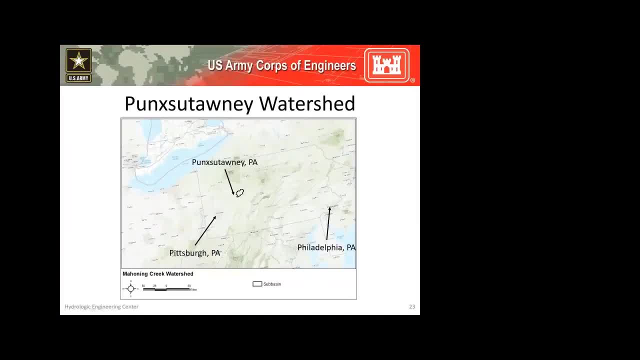 Punxsutawney- West. Punxsutawney is on Mahoning Creek, Which is a tributary to the Allegheny River, which comes together with the Monongahela to form the Ohio and Pittsburgh right. So Punxsutawney is just on the downstream end of the modeling domain. that. 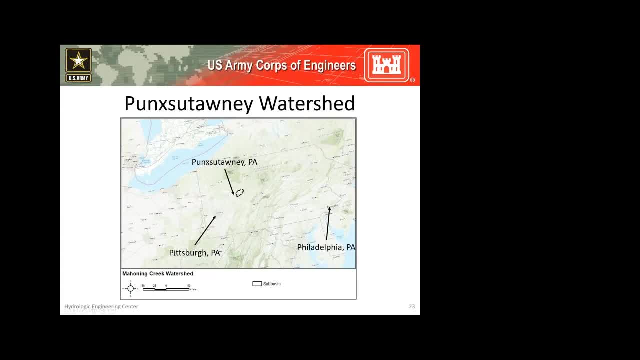 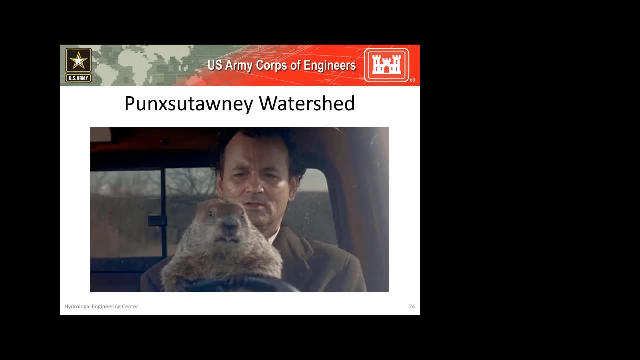 we're talking about in black. If you aren't aware of it, this is where Groundhog Day took place- Great Bill Murray movie from 1993.. I can't believe it was that long ago. I love this movie. It's a. 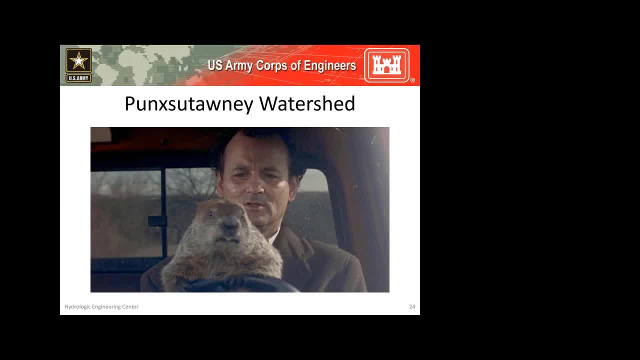 great one. Quotes from this movie will be in the final exam, So if you haven't watched it in a while, definitely take a look at it. Just keep an eye out for that And I'll see you next time. Thank you. 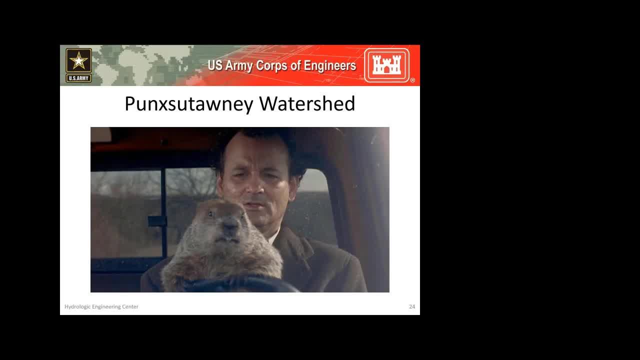 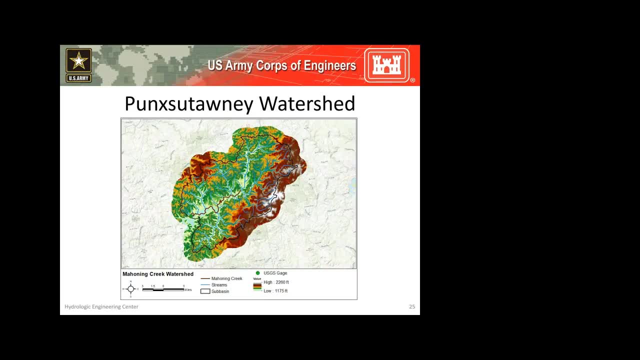 I'm not sure if there's a book that accompanies that or not. A little bit of background on the Punxsutawney watershed. There's a gauge there at Punxsutawney on Mahoning Creek. That's about 158 square miles. It drains to it. Elevations range from about. 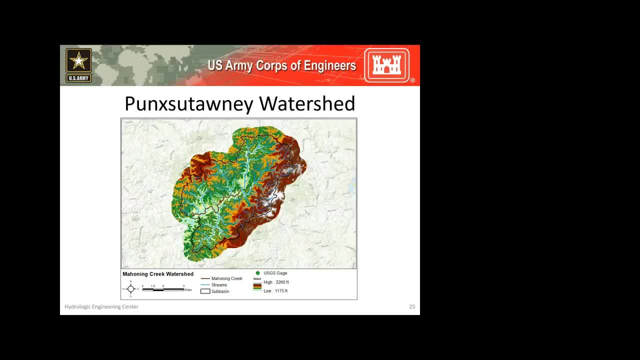 2,260 feet to 1,175 feet. So that picture that you saw at the beginning. there is not that much elevation change here in the Punxsutawney area, Definitely, definitely not taking place. That picture is from the Punxsutawney watershed. There's not that much elevation change here in the 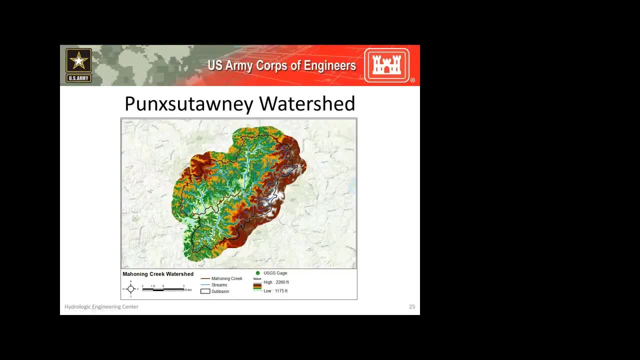 Punxsutawney area. Definitely definitely not taking place. That picture is from the Punxsutawney watershed. Definitely definitely not taking place. That picture was not from Pennsylvania. There are some major tributaries. Stump Creek comes in from the north, So this is Stump Creek. 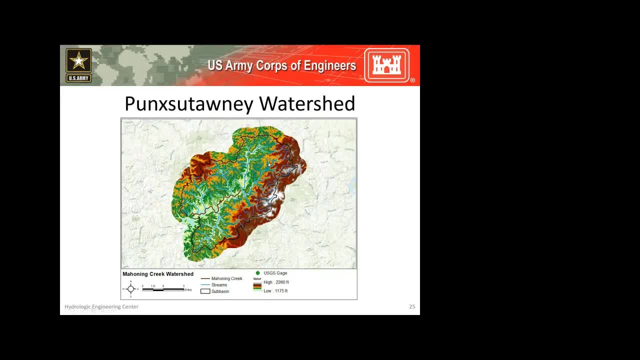 where my mouse is going, East Branch, Mahoning Creek kind of comes in from the south, from the east. whatever, Those two come together and form the main stem, Mahoning Creek, which flows through Punxsutawney itself. You guys will be dealing with this in a couple of different iterations. 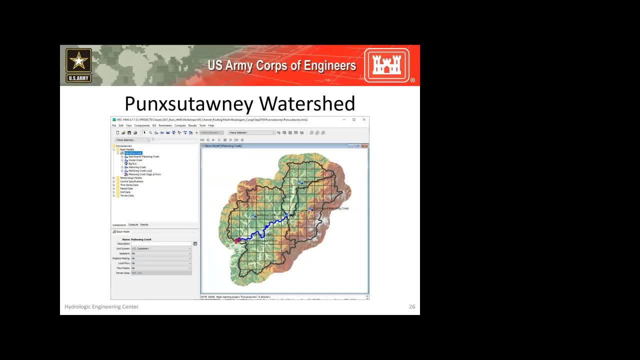 Sometimes you'll be looking at it in HMS, where it's just a single subbasin That 158 square miles, just one subbasin. Other times you're going to be looking at it with three different subbasins. Become familiar with this. Look at the different setups. You guys will compare and 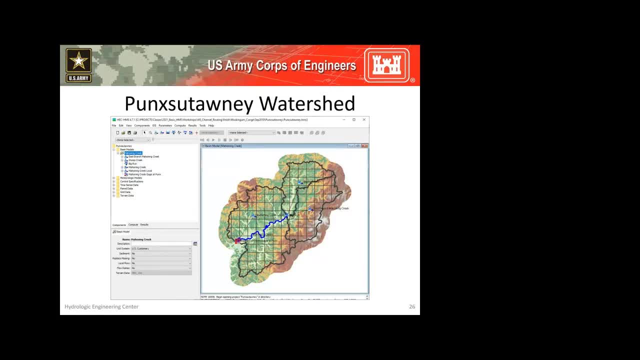 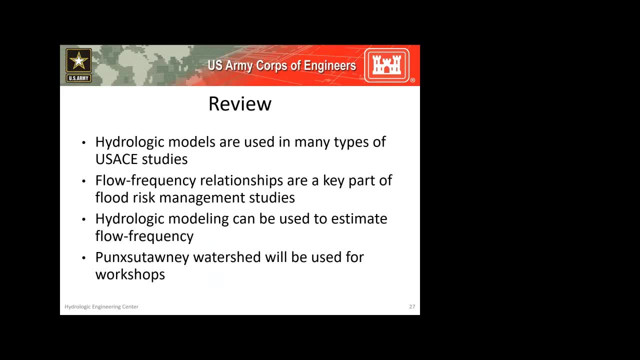 contrast them as you go through as well, But this is generally how the watersheds will line up within HMS. All right, so quick review and then we'll be done with this one. We can go to one of our breakout rooms. Hydrologic models are used all throughout the Corps. Hopefully you guys are.